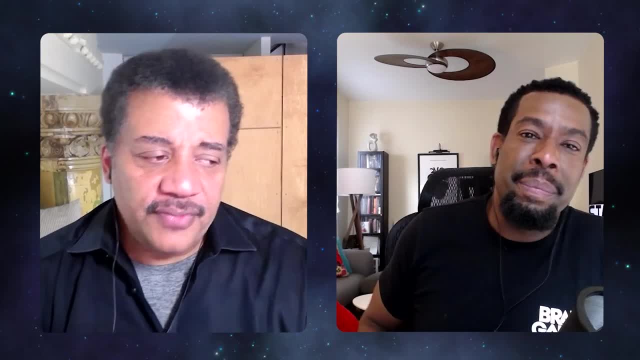 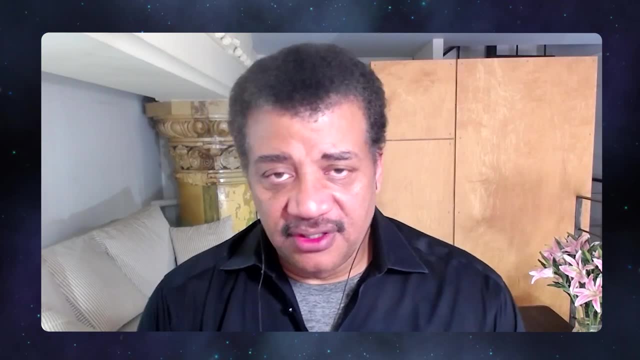 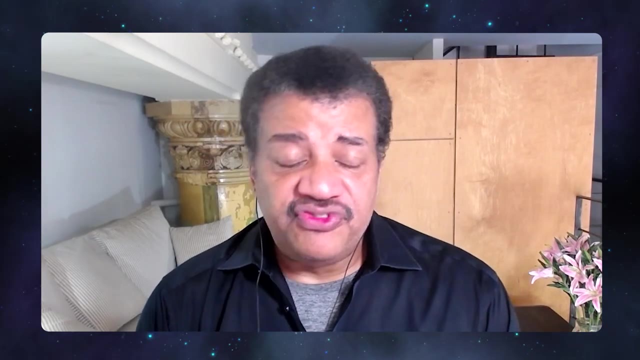 I'm sorry, All right, So before we pick up wavicle, let me just remind you that light, which in my field we call the electromagnetic spectrum- Okay, Is all forms of light Most familiar to us is visible light, Okay, Red, orange, yellow, green. 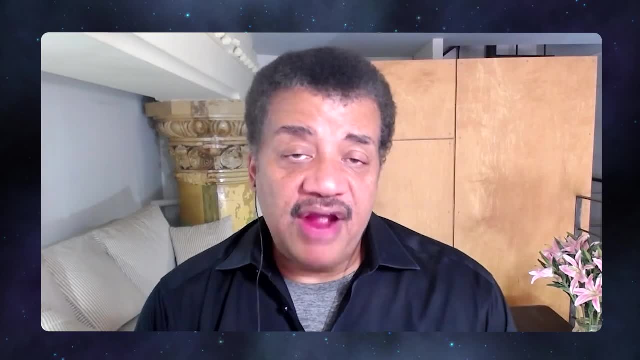 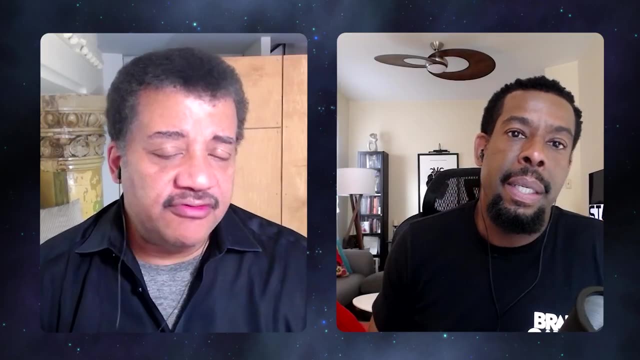 blue, violet, Okay, But if you go on the other side of red, you get to what? Infrared? Infrared, Very nice. Your retina can't detect it, but it exists. Right, We do have infrared sensors. We detect it on our skin as heat. 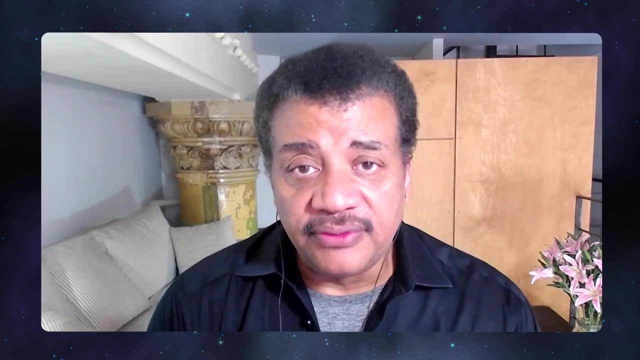 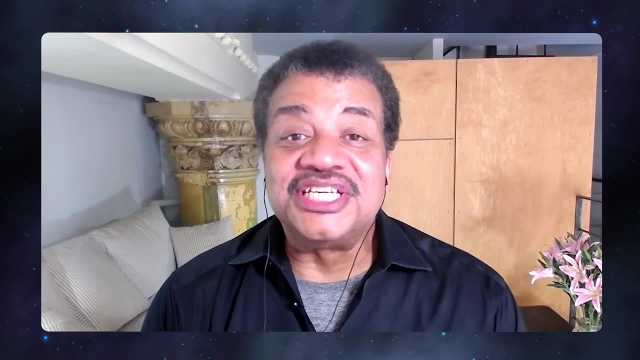 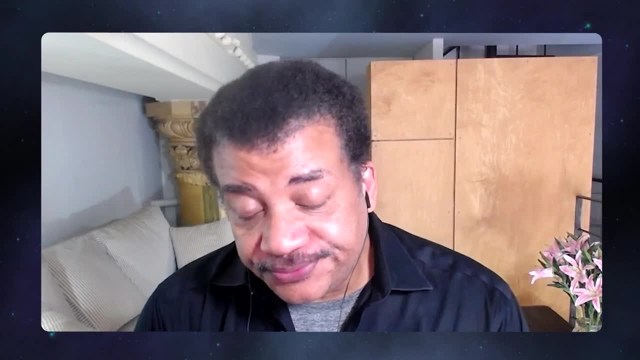 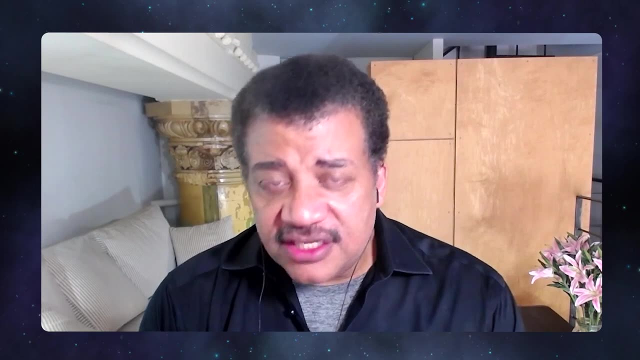 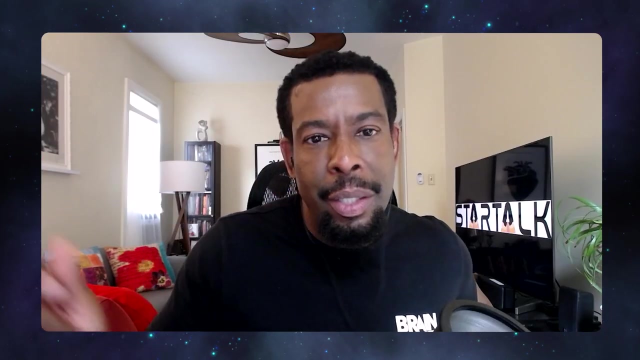 Okay, Now you go beyond the violet. you get what? Ultraviolet, Ultraviolet. so that's beyond the violet. We can't see ultraviolet either. We also have sensors for ultraviolet, but they're significantly time delayed. Oh, I thought you meant like black lights that just show us all the nastiness that happened in a hotel. 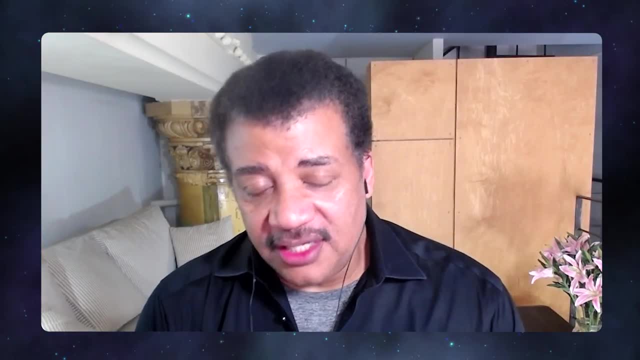 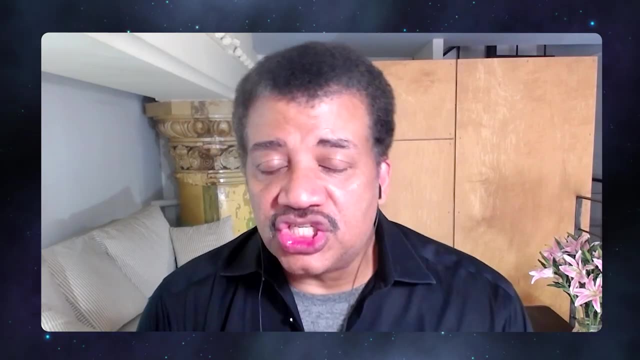 Oh, no, no, no, That, no. what happens in the in under blacklight is you're illuminating the crime scene with ultraviolet lights, ultraviolet light which you cannot see, and certain substances fluoresce under it and send you the. 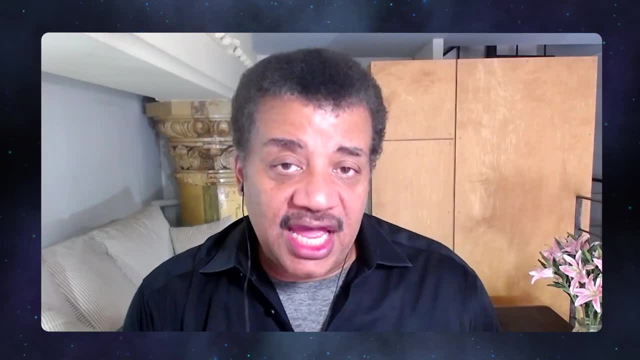 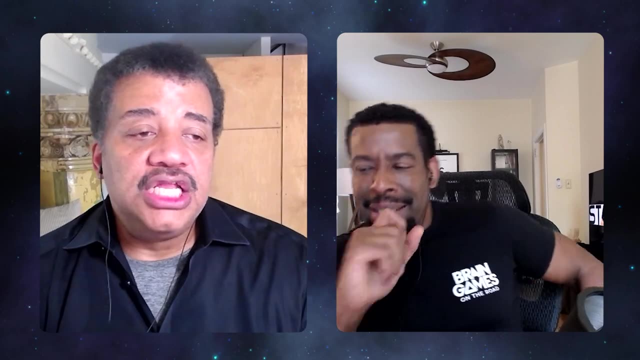 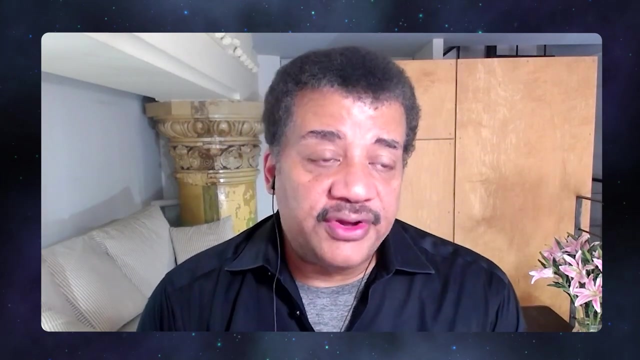 light back in violet light that you can see. so you're never seeing the ultraviolet. you're never seeing the ultraviolet. no, no, no, no, no, no, okay. so so here we are in ultraviolet. we have ultraviolet sensors. they're just time delayed, okay. okay, the time delay is okay, you're out in the sun. 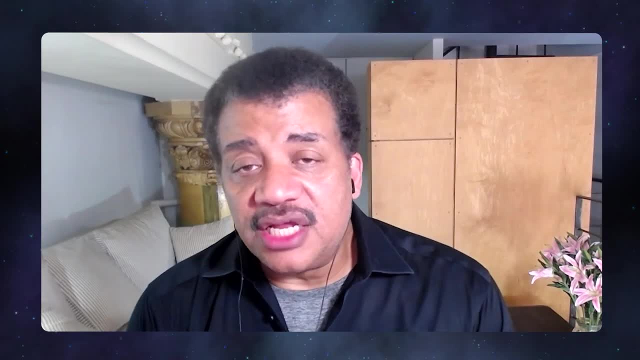 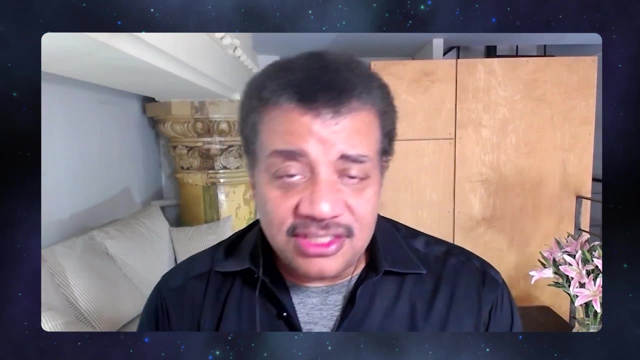 oh, and an hour later, you feel like you have your sun. if you have lighter colored skin, you're, you feel like you're, you get sunburned, and you do that enough, then you get skin cancer. these are, in a way, detectors of ultraviolet. it's just too late, right, okay, right, all right, let's go back the other end. 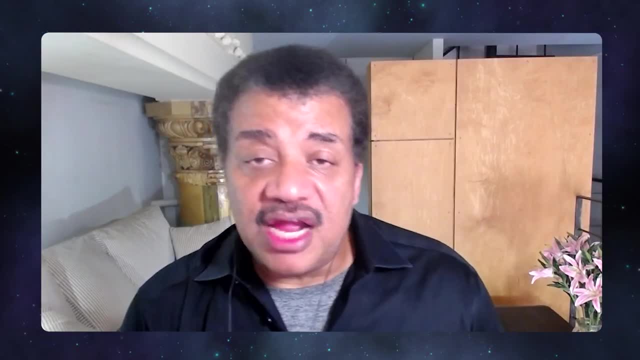 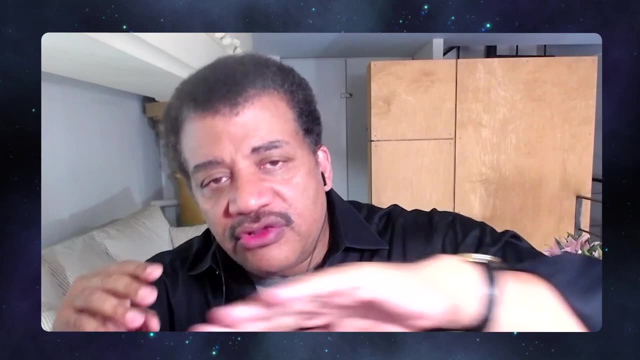 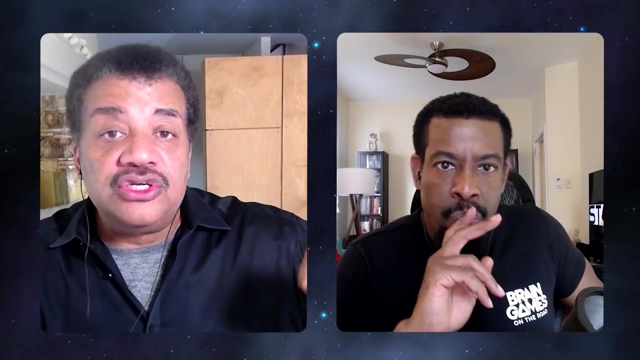 uh, so we had red infrared and you keep going in that direction on this spectrum. by the way, what's changing on the spectrum is the wavelength of the light. okay, so as we go to the red, wavelengths are getting bigger and bigger. we get to ultraviolet, we get to infrared. beyond infrared, we get to microwaves, micro, yeah, okay. so now i can describe. 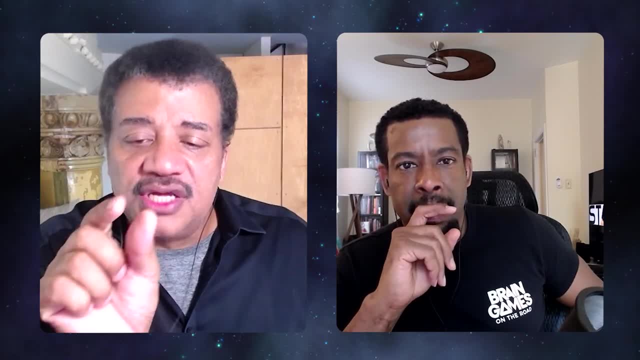 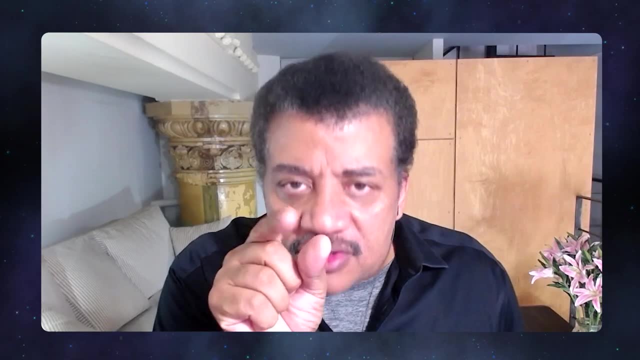 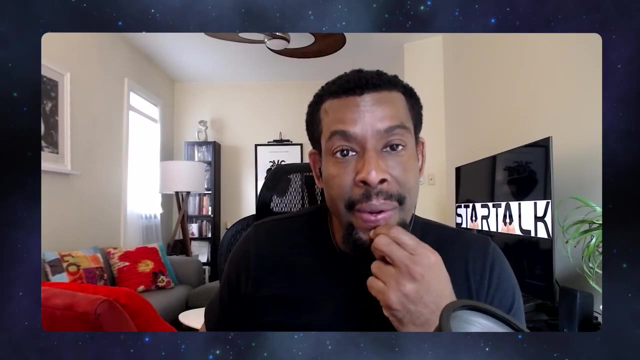 the length of the wave, like with physical fingers and things. so a microwave is like a few millimeters to like maybe a couple of centimeters around. wow, let's just call it a centimeter. yeah, a physical centimeter that's. that's a pretty big wave. that's a big wave. that's a half an inch and so, wow, full. 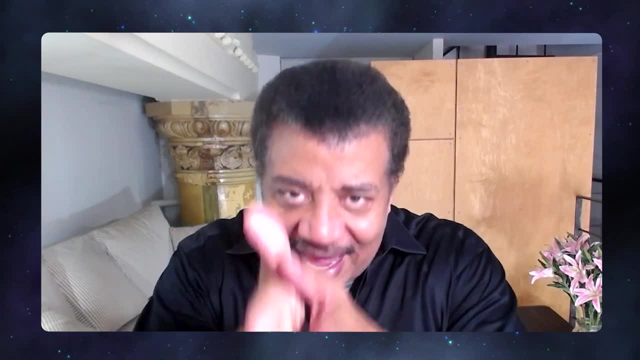 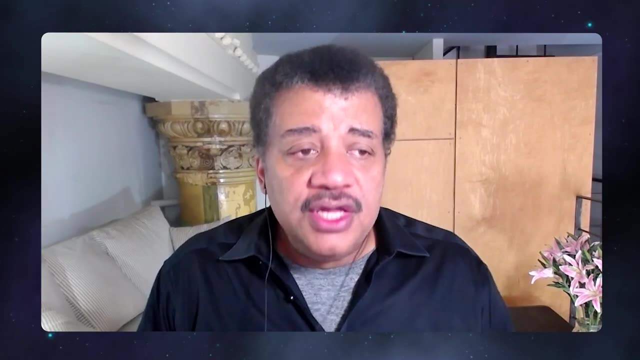 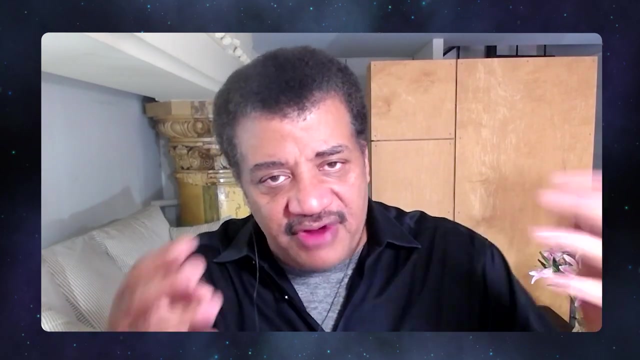 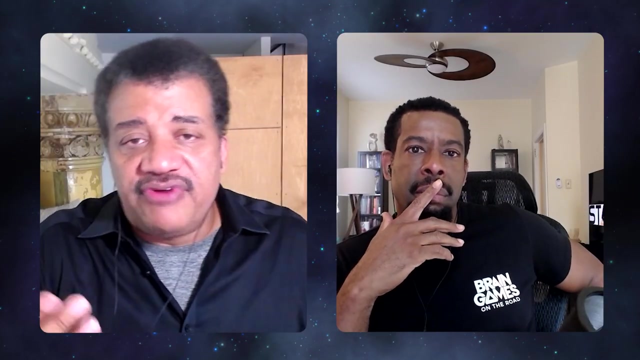 wave, a crest and a trough gets manifested in that space. when you have microwaves, okay, nice, okay, let's go beyond that. you get to what we call radio waves, right? so before microwaves had their own name, they were just short wavelength radio waves. okay, you've heard shortwave radio? yeah, okay. so then we said: well, there's small versions of 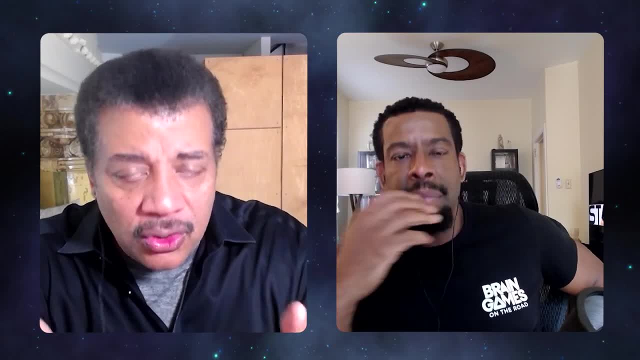 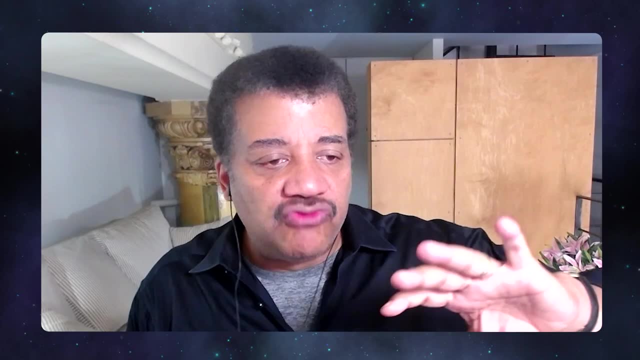 radio waves, let's call them microwaves, and that's why they're. they're called micro, even though they're bigger than infrared, right, all right, that's all i'm saying here, okay, so? so radio waves are like meters and longer. we don't have words. a radio wave can be. 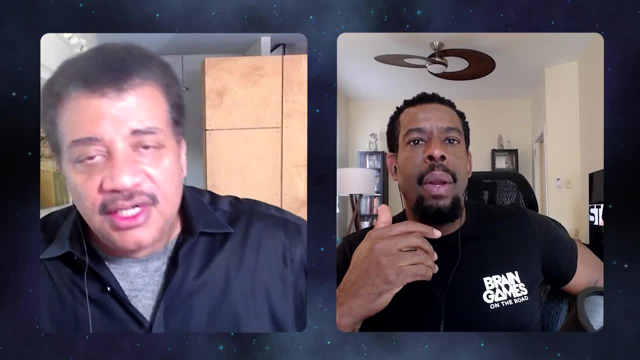 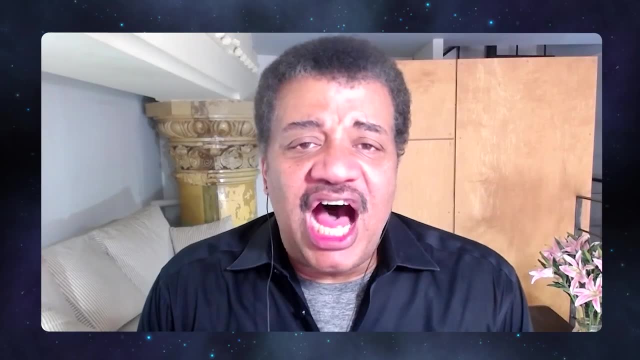 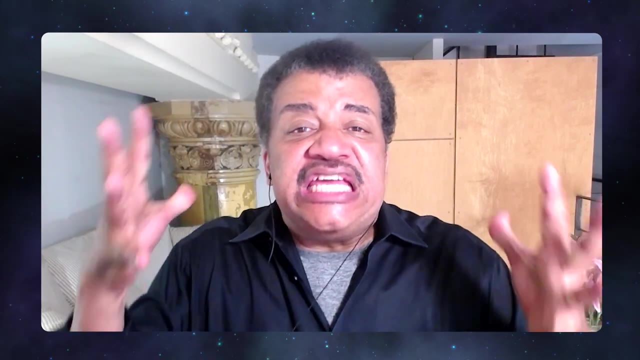 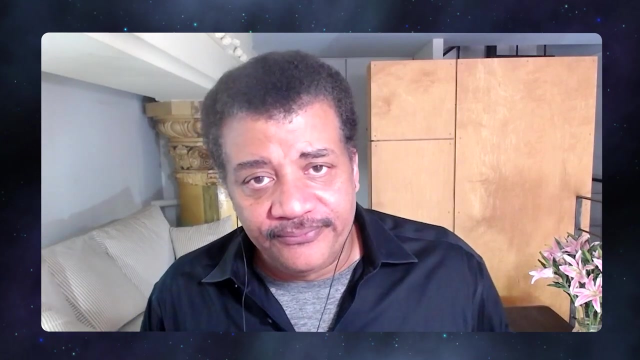 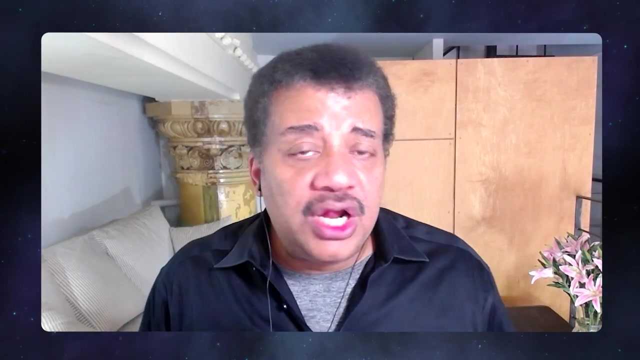 miles in wavelength. we don't have a different word for that. so radio, radio waves are for everything bigger than microwaves. all right, so now watch. if i want to detect a radio wave, i need a thing that's at least as big as one of the waves- gotcha. so tv, old world tv- before it came in via cable, used antennae. 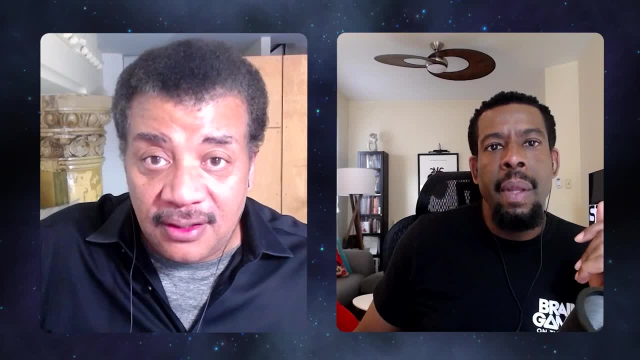 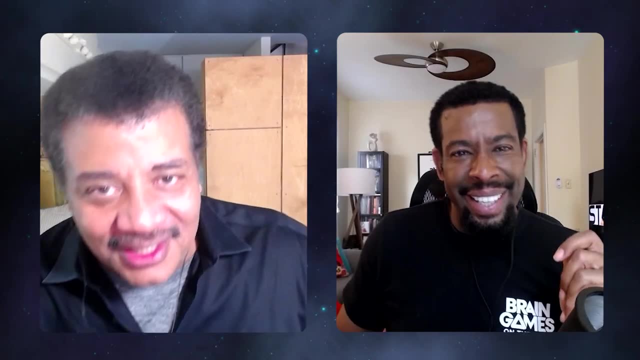 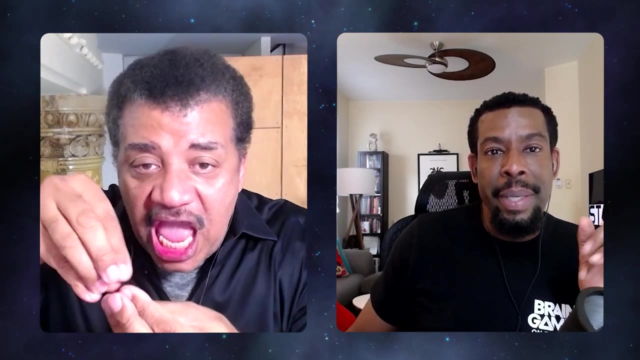 how long was a tv antenna? um two stories high. the one on your tv exactly was about a meter long. right, yeah, okay, in fact you'd have two of them sticking out all over the place and you'd extend it to about the length of the waves of the, of the. 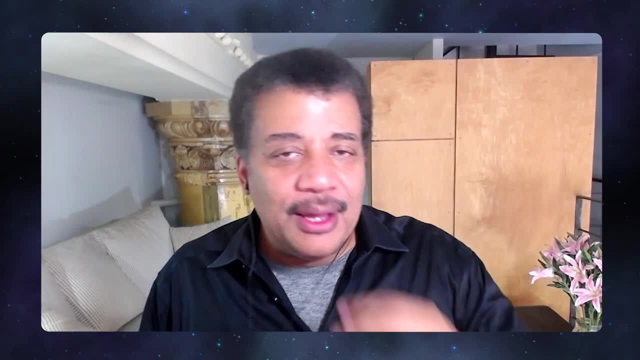 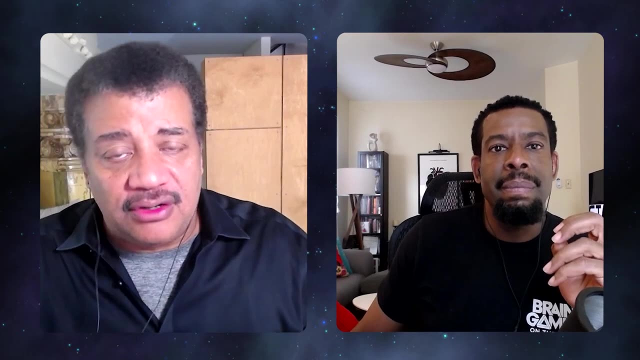 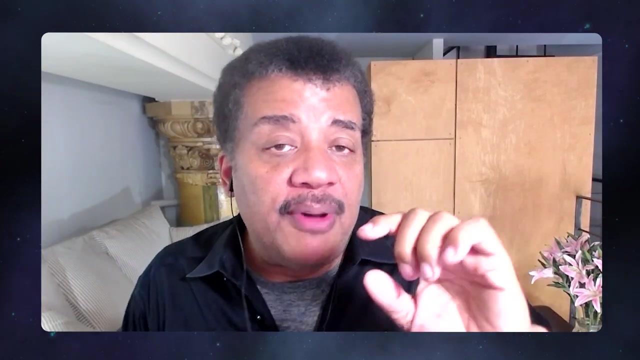 radio waves you're trying to receive. okay, all i'm saying is: you can't detect waves bigger than the size of your detector. it doesn't work, okay. okay, it'll just wash over your detector and your detector won't even know what happened, right? so how about microwaves? have you ever seen a microwave? 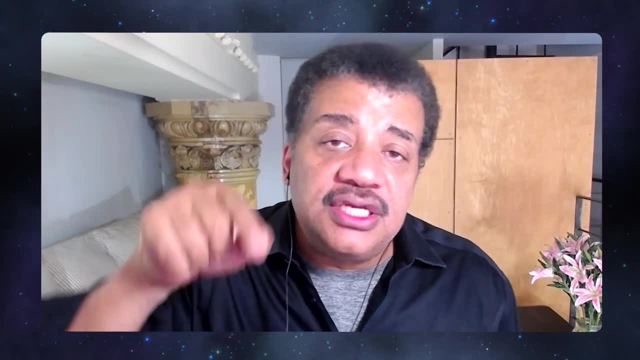 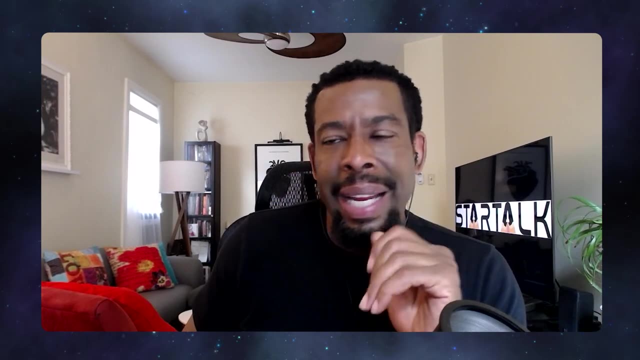 um walkie-talkies. i've never seen a microwave walkie-talkies. i've never seen a microwave walkie-talkies. how long is the antenna on a microwave walkie-talkie? uh, you know, it's about like that. there's nothing to it, it's about. it's about it's like an inch and a half. there's your microwaves. 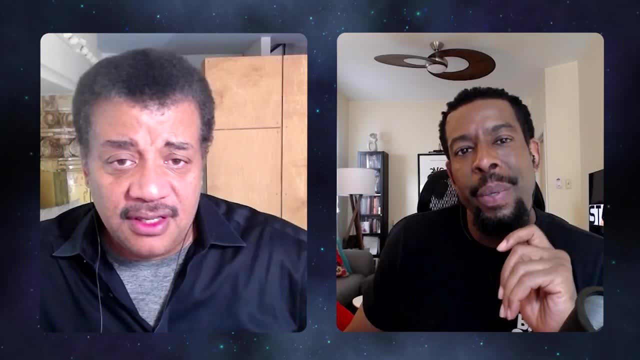 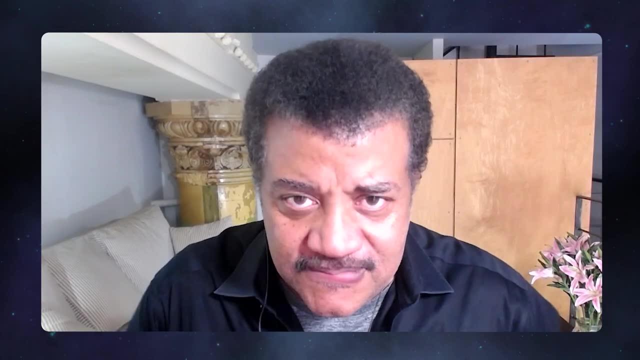 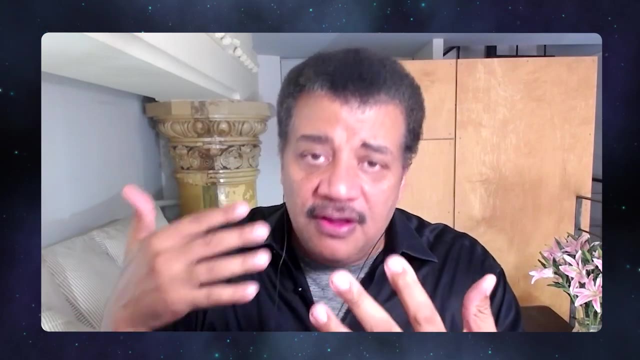 that's the size of the microwaves. that's pretty wild. that's, that's so it. it is the size to fit the situation right. okay, that also means if you have a substance that prevents the transmission of a microwave walkie-talkie, you're going to have a microwave walkie-talkie. 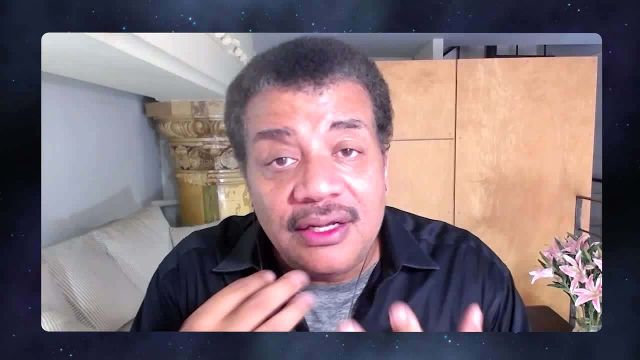 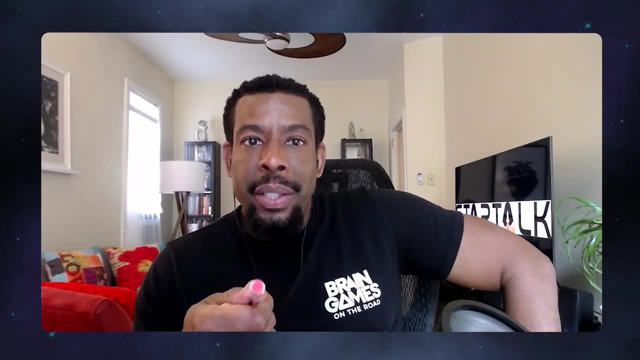 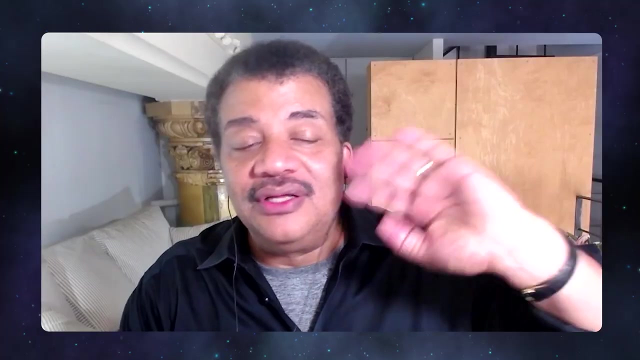 okay, you could put holes in it, and as long as the holes are smaller than the wave, the wave is not going to get through. whoa, that is that the like. so take a look at your microwave oven. that's what i was about to say. that's why all the black ways, so white microwaves go through glass, no problem. 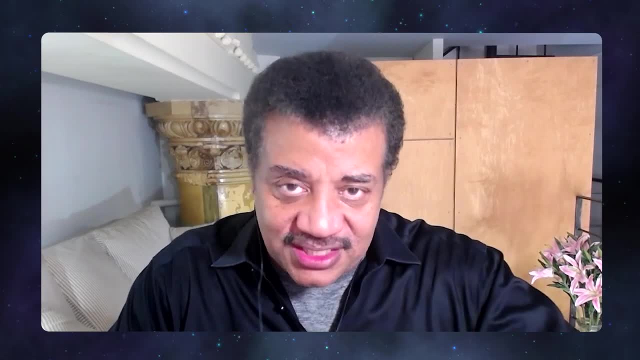 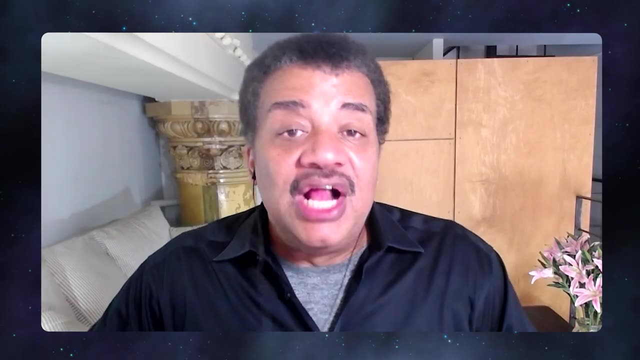 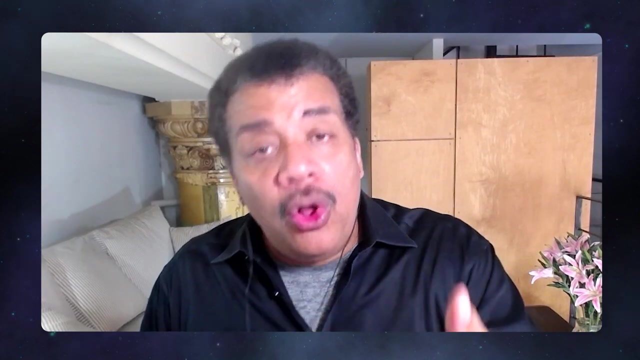 gotcha. all right so. but so you have a glass thing so microwaves and visible light go through so you can see your food cooking. but there's something else. on the other side there's a screen screen, yeah, and that screen is opaque to microwaves- okay, except they put holes in it. now, that's why i got. 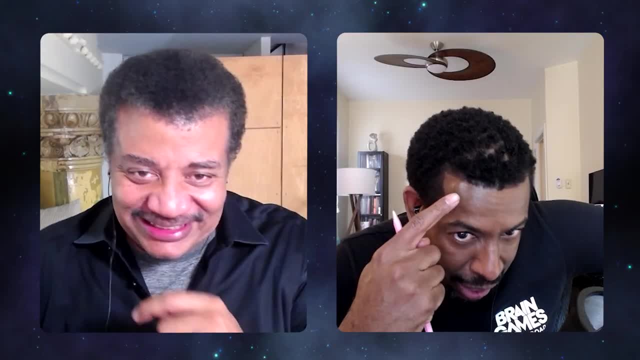 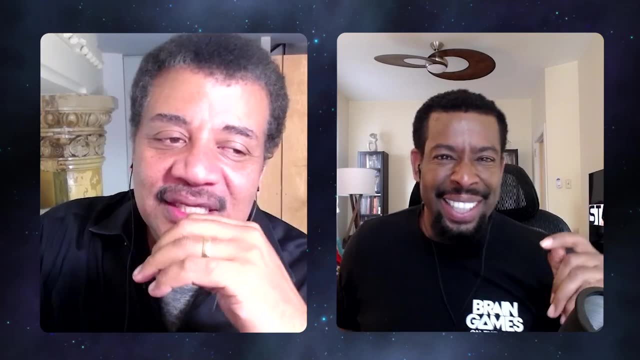 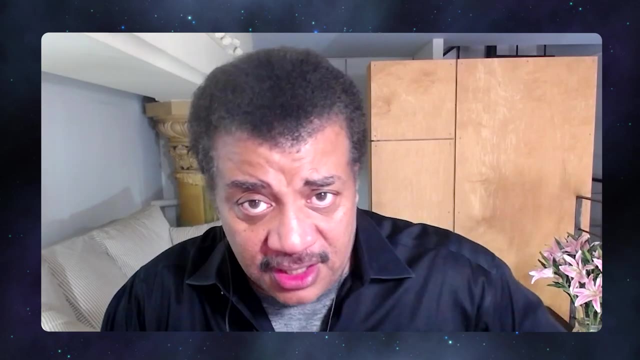 this tumor on my head, don't you stop? is that? why don't stick your hand inside the microwave, so so neither you nor the microwaves can see through that material, except for the fact that they put holes in the material right. how big are the holes? 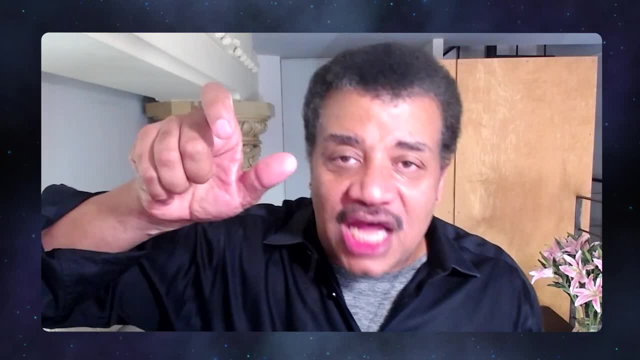 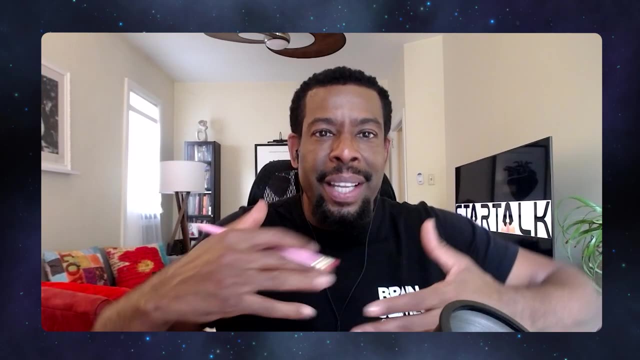 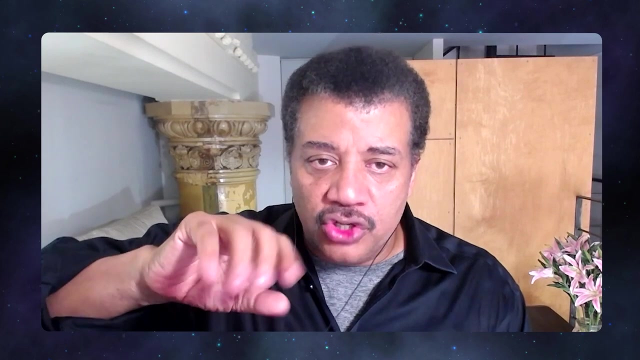 tiny. they're smaller than the size of the microwaves they're using in that oven. that's pretty wild. microwaves cannot. it's the antenna in reverse. in reverse. oh, i like that very clever, cool, clever. so so so you can put holes in things. so radio telescopes: have you ever seen a radio? 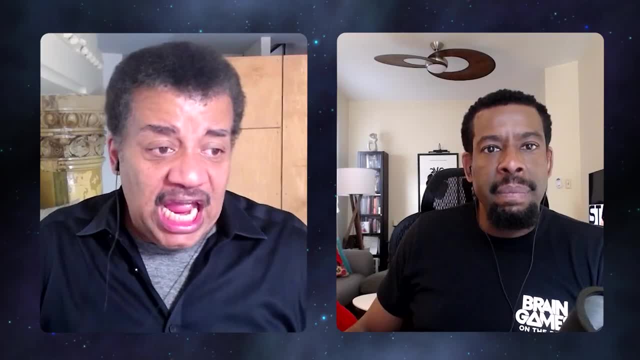 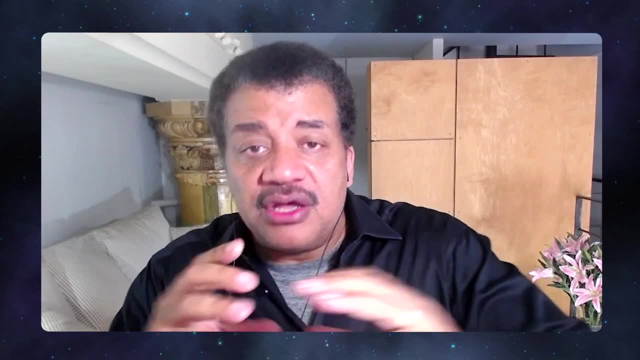 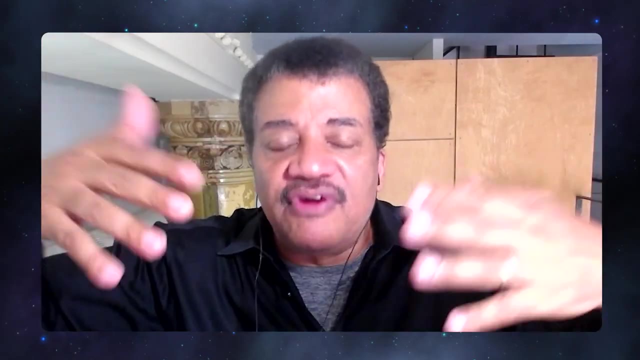 telescope go to a radio telescope one day. they're huge and they're made of like mesh. they're like chicken wire- mesh mesh, with these huge holes in it, because it's the- depending on which kind of radio telescope you're visiting- that the, the metal, is reflective of radio waves. but you don't have to build the. 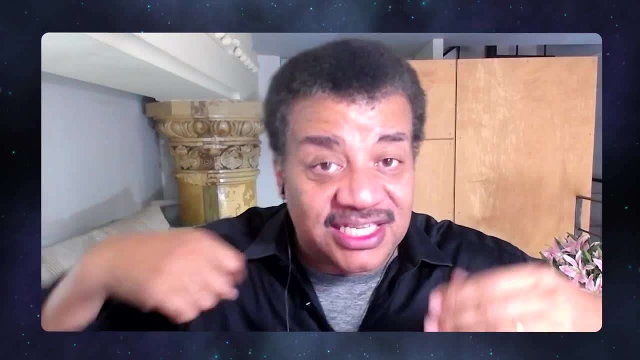 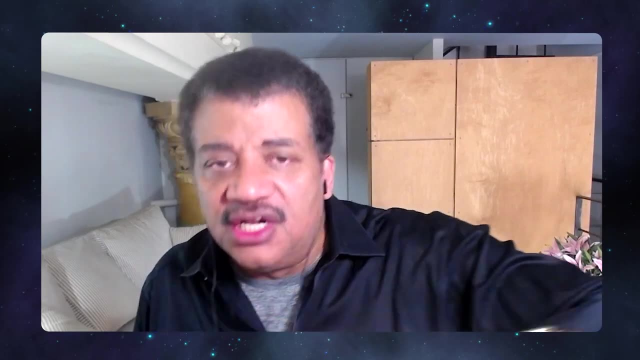 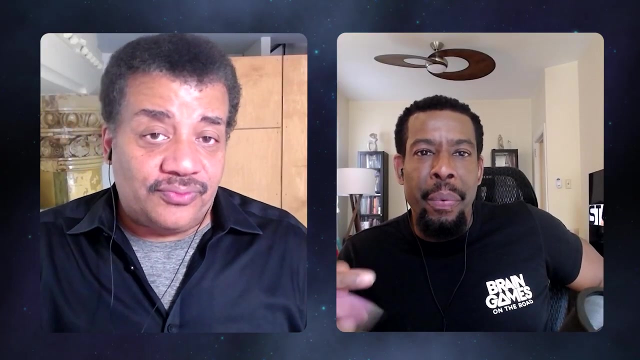 whole surface of metal. you can put big holes and it makes it lighter, all right, and rain can get through and not a problem. and with because of these huge dishes and they can take radio waves, reflect them to a focus and there you have it. that is a really really 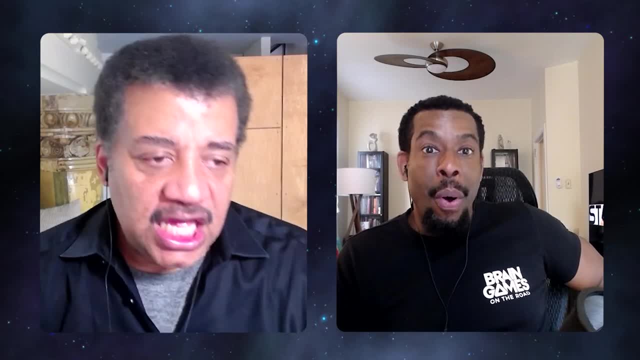 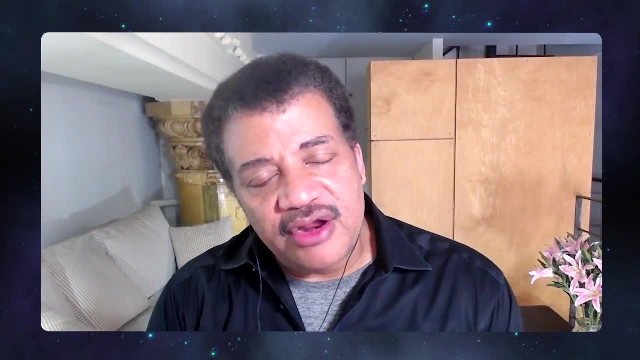 cool. well, let's keep going in the other direction. oh, okay, okay, there's more. well, wait, there's more. okay, i was satisfied. but yes, please consider, let's go the let's go the other direction. so we go: red, orange, yellow, green, blue, violet ultraviolet. you go beyond ultraviolet. you have x-rays, x-rays. 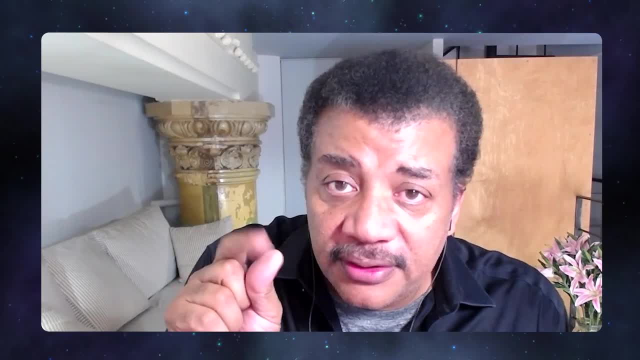 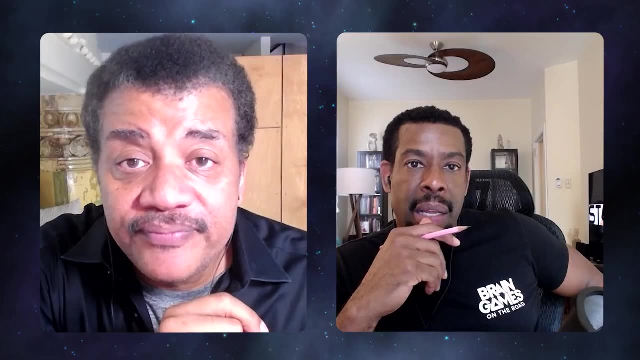 wavelengths are getting smaller and smaller and smaller and smaller. okay, really, tiny, tiny, tiny tiny, much smaller than the wavelengths for visible light. aha, all right, so now watch. if i have a regular microwave, i'm going to put a little bit of light in there and i'm going to put a little bit. 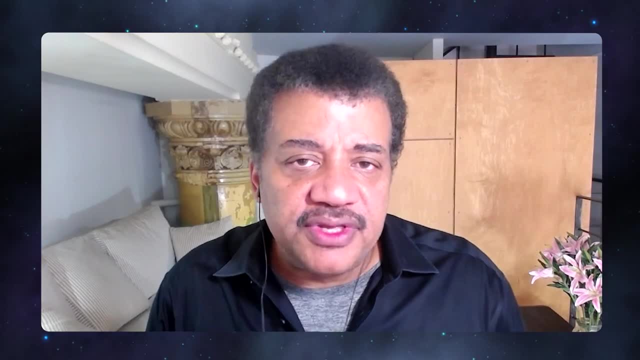 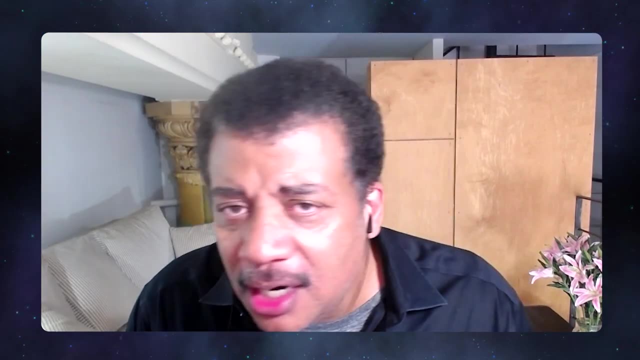 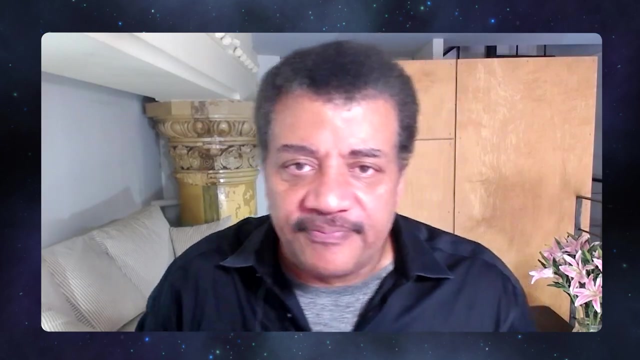 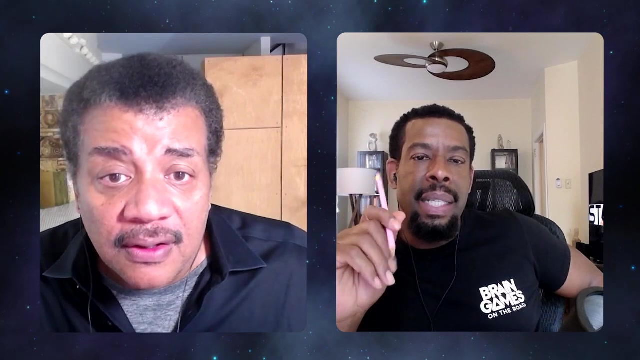 of a microscope and i want to see something small. i cannot see anything smaller than the wavelength of the violet light i'm using in the visible spectrum, oh man, because otherwise it washes right over. it would not even know it's there, right, okay? so if you want to see things smaller, 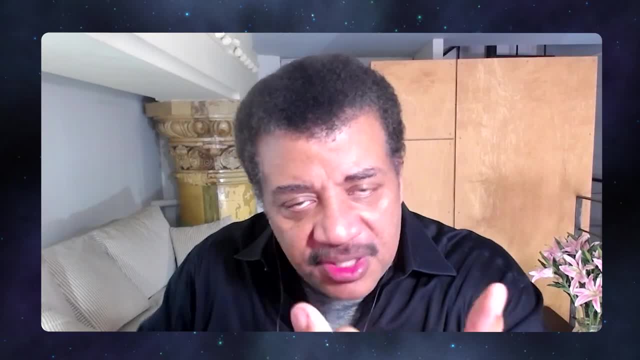 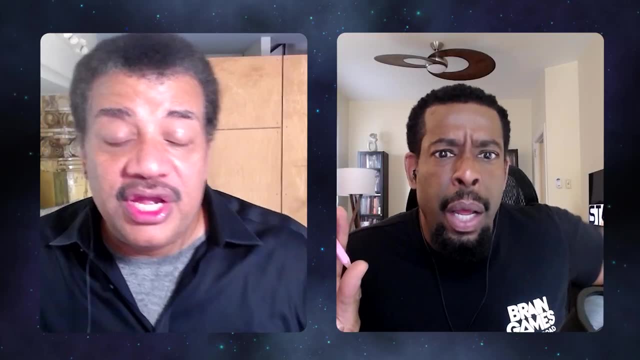 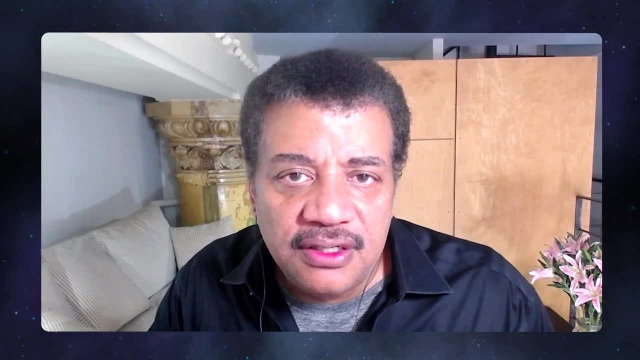 than the wavelength of the violet light. i'm using in the visible spectrum, the wavelength of visible light. that would be the violet side of it. you need even smaller wavelengths of light, interesting so. so here's talk about getting clever. you ready, okay. so people said, how about electrons? right, you say. well, electrons are particles. they're not waves, they're also waves. 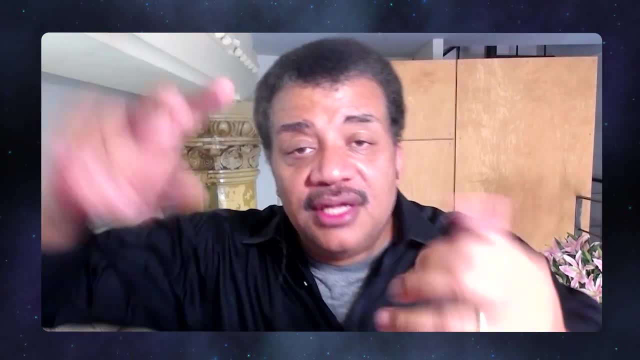 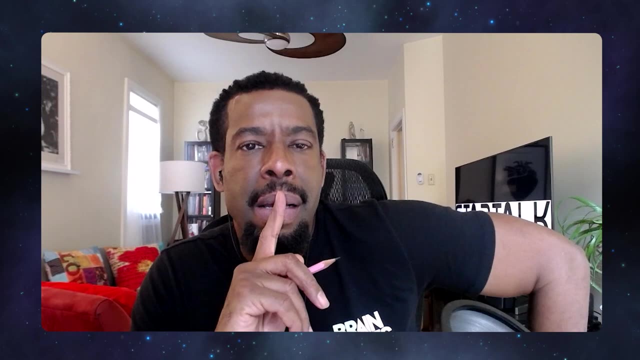 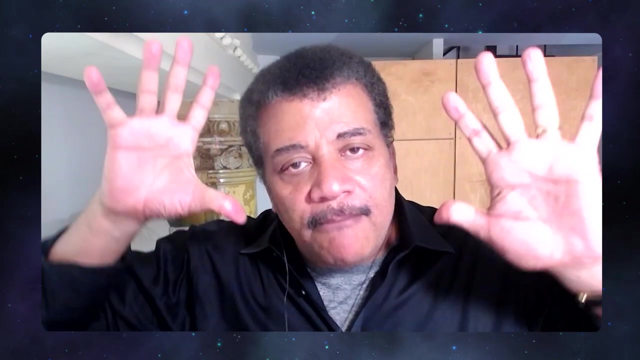 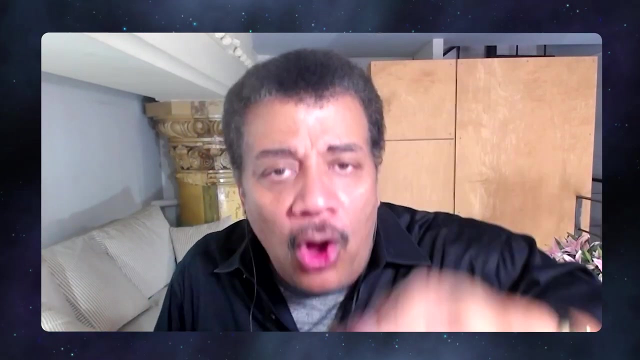 oh my gosh, what wavelength corresponds to electrons that we could generate in the machine- x-rays. oh my gosh, so electrons and x-rays have the same wavelength? wow, so if i invent a microscope that uses electrons, then i'm using a wavelength of light as small as x-rays, so i can see the. 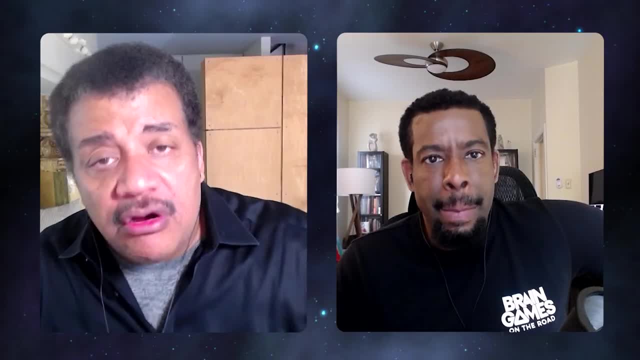 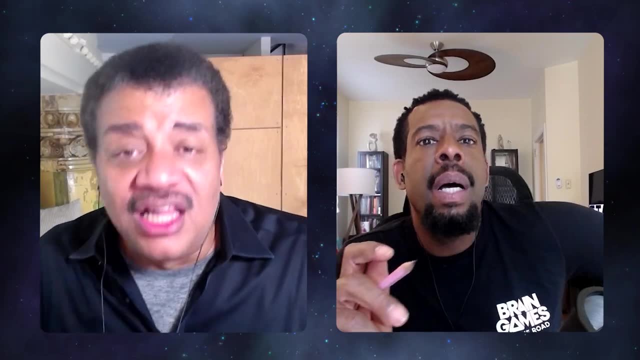 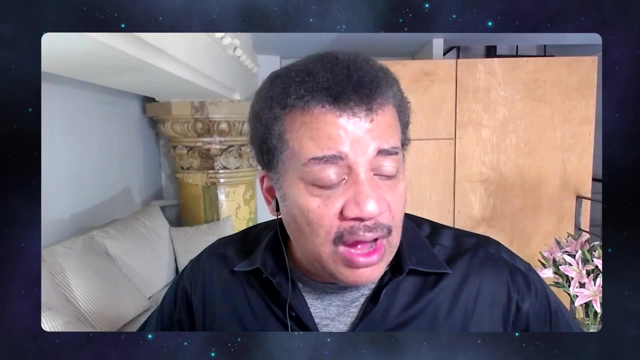 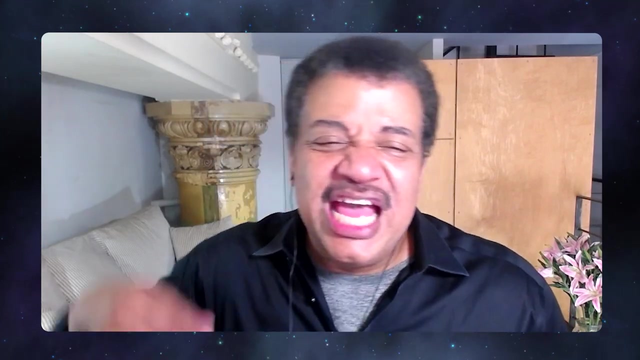 tiniest detail. so the photographs that have this, the most exquisite detail of the smallest things, are not regular microscope photographs. they're electron microscopes because we, we quit, we, we- what do you call it? we co-opted, we commandeered electrons, piggybacked an electron using the x-ray wavelength that it represents. 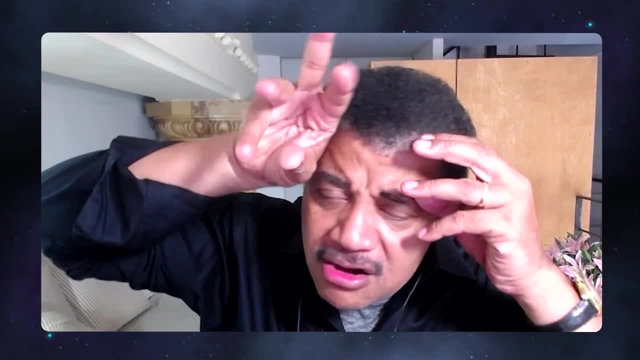 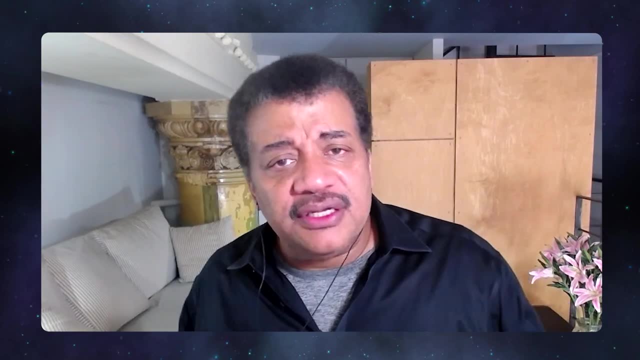 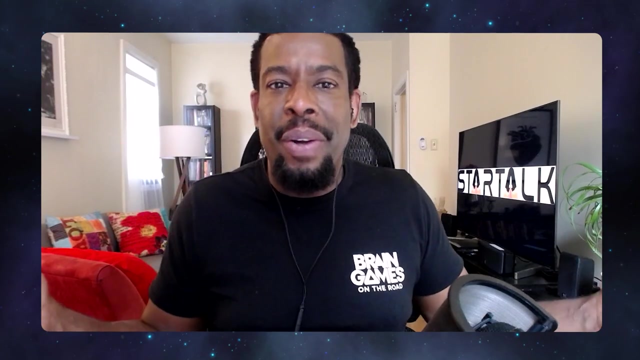 to take. that's why you see those bug pictures with the hairs and the thing, yeah, and and, and, and the, the bacteria, all this. there you go. that is fascinating, that that's. that's, that's how electron microscopes work. that's how they were, isn't it? 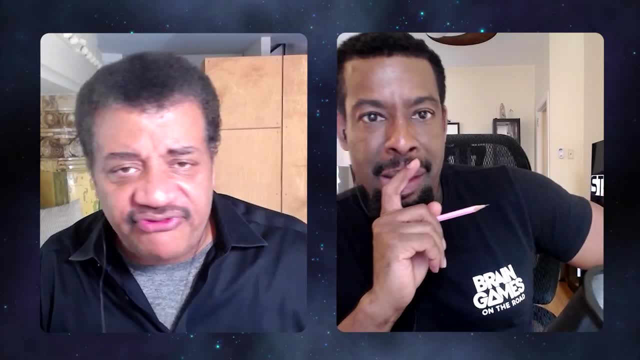 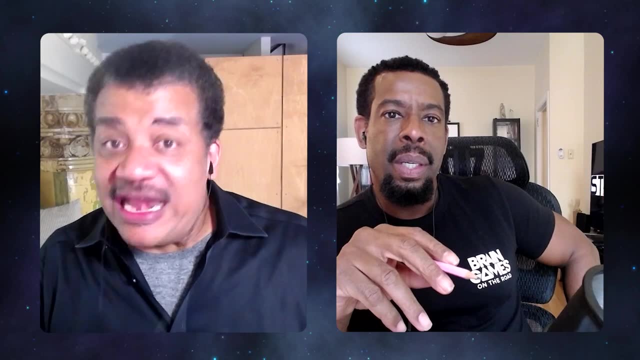 clever of the human mind to do that. after quantum physics we said we got the wave particle duality, and i can't see anything smaller than the wavelength of violet light. but i know there's got to be detail there, because there's detail up until the point where it gets fuzzy, right. well, let. 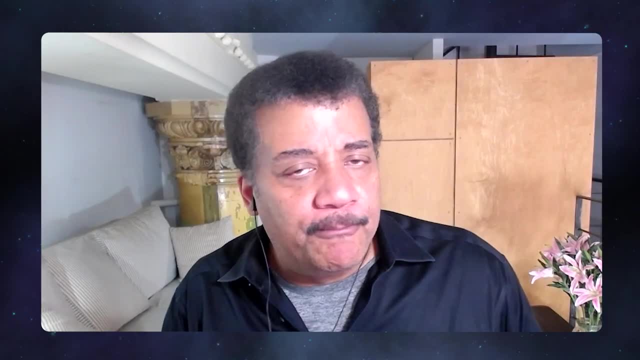 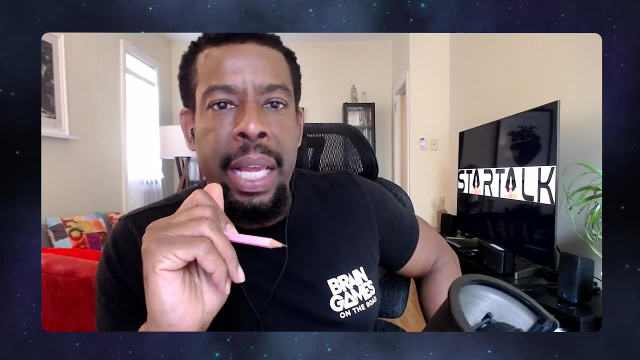 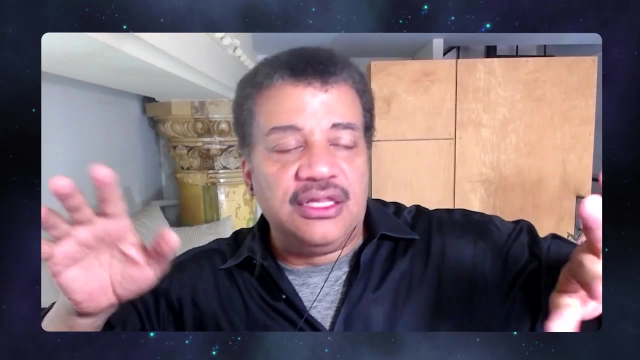 me keep going. and then you invent the electron microscope and bada bing. the world of of the small continues to open to you. so that means, if so, is our gamma. what's the smallest wave is a gamma. so the smallest uh waves that we have a word for are gamma rays. so gamma rays are like, are the? 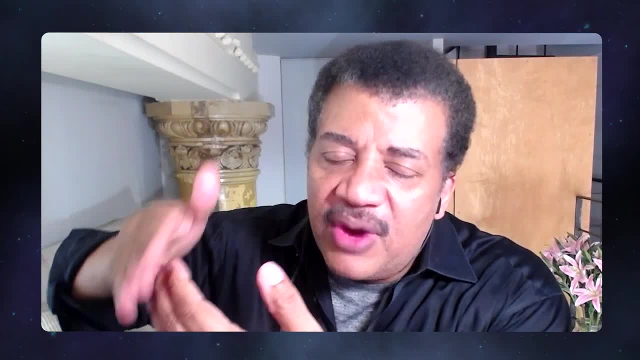 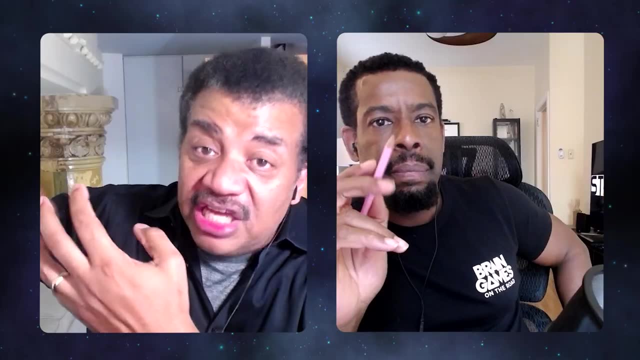 opposite, like like radio waves- so it's smaller wavelengths than x-rays- are gamma rays, and then we don't have it, we don't keep dividing it, so, so gamma rays that are like really, really, really small, they're still, they're still called gamma rays. yes, okay, gotcha. so the problem is, if you 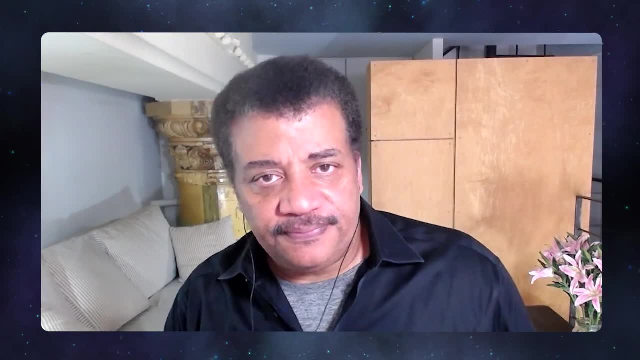 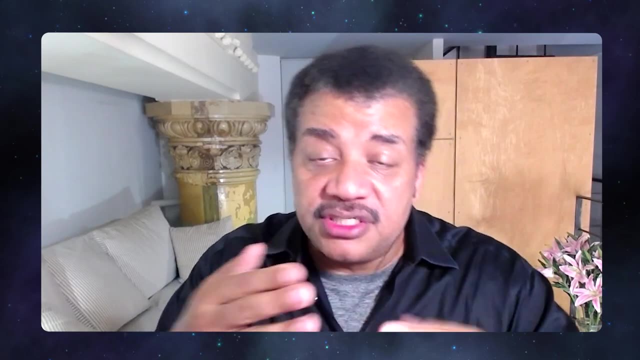 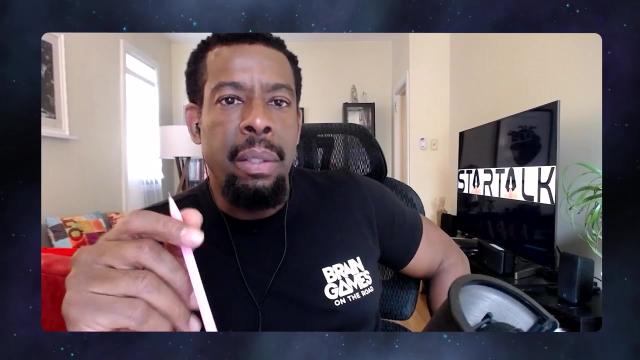 a gamma ray telescope, you have to be able to focus it. okay. it's not good enough just to use the light you have. you need to be clever about when the machine you're making and we know how to focus electrons because they have a charge right so we can focus them down and get images and things. so yeah, so the only thing, uh.